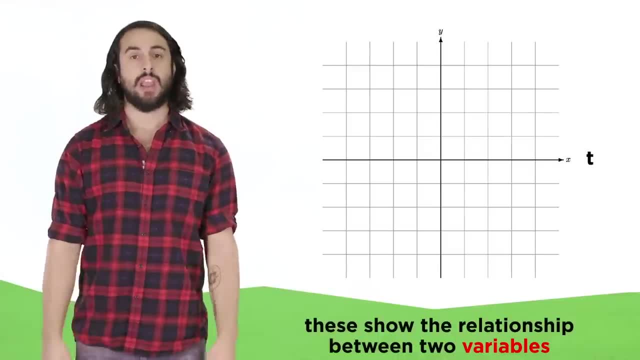 So we can label the X axis with a T for time and we could make tick marks for individual seconds or multiples of ten seconds or whatever we want. On the Y axis we will put some other variable and right now we want to learn what happens. 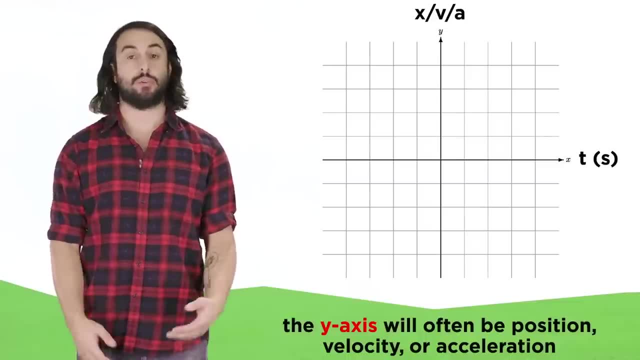 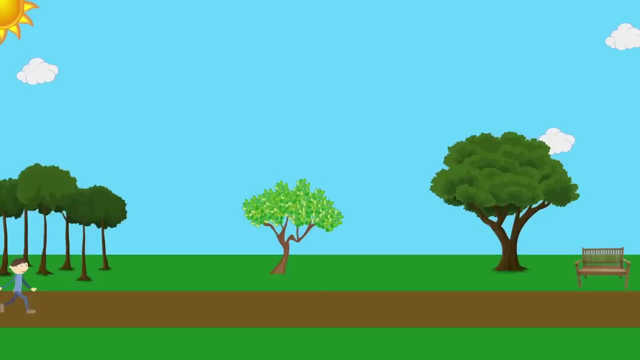 when this variable is position, velocity or acceleration. Let's go through an example and generate all three of these graphs. Say you are walking on a path in the woods on a fine autumn day. You walk the one kilometer path at a rate of one hundred meters per minute. all the 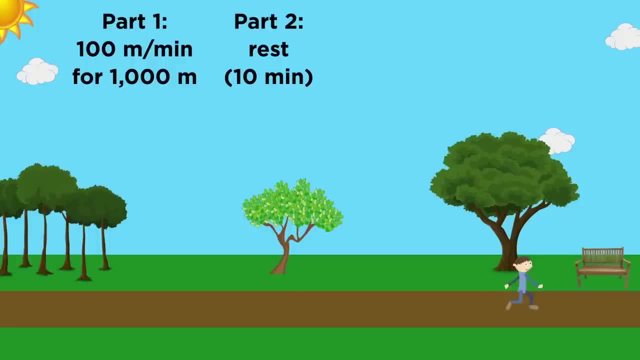 way to the end of the path. Then you sit and rest on a bench for another ten minutes thinking about what to have for lunch. Once you've got an idea, you get very excited, so you begin to run back the way you came. 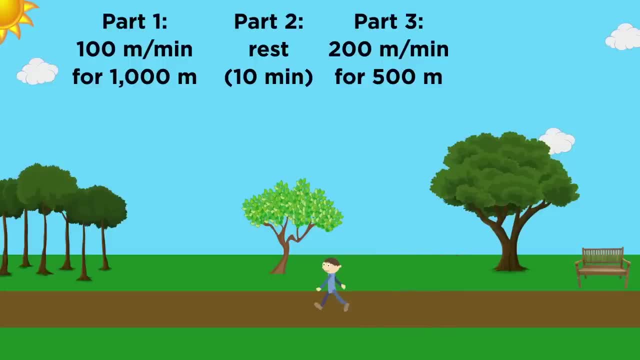 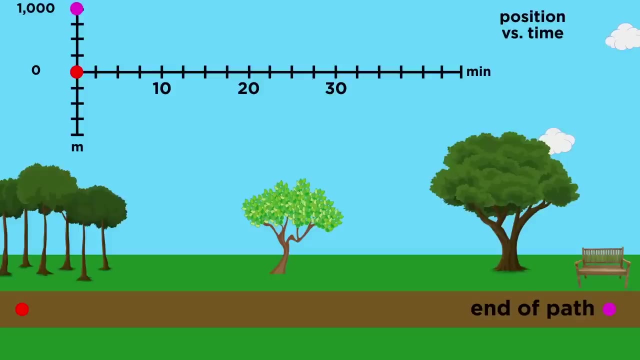 at a rate of two hundred meters per minute, But after you get halfway back you become tired and you slow down to fifty meters per minute. Let's represent all of this on a graph of displacement versus time. If the point where you started is the origin, and this point on the Y axis is one-third, 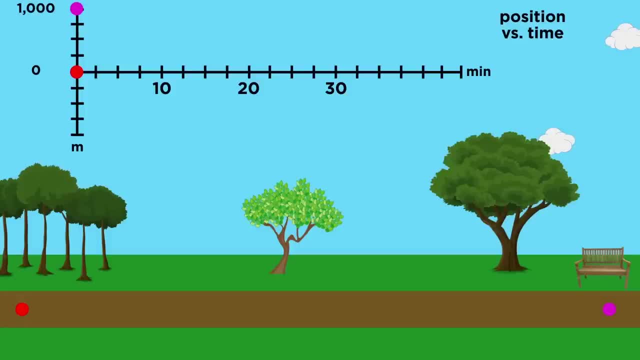 is one thousand meters where the bench is. we can draw lines to represent each section of your walk. First you went the whole kilometer at a speed of one hundred meters per minute, so over ten minutes you went a thousand meters. This line represents that activity because it goes from the origin, the beginning of. 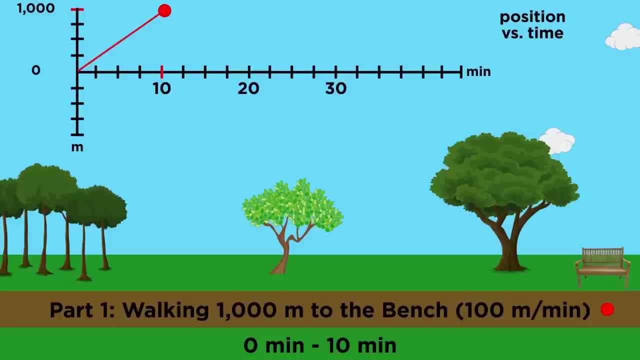 the walk to a point with coordinates of ten minutes and one thousand meters. Be sure to understand that this line does not represent a path in two dimensions. All the motion is along one line, but you are also moving forward in time, and that's. 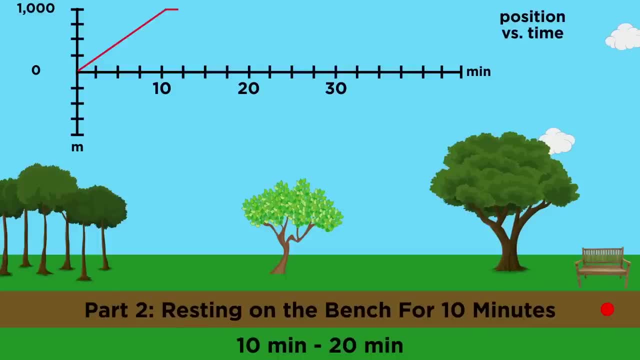 what the X axis represents. Now you are at the bench and you sit and look at the trees for ten minutes while thinking about snacks. This means you will move forward in time by ten minutes, but your position will not change. so this is represented by this horizontal line segment ending at a point with coordinates. 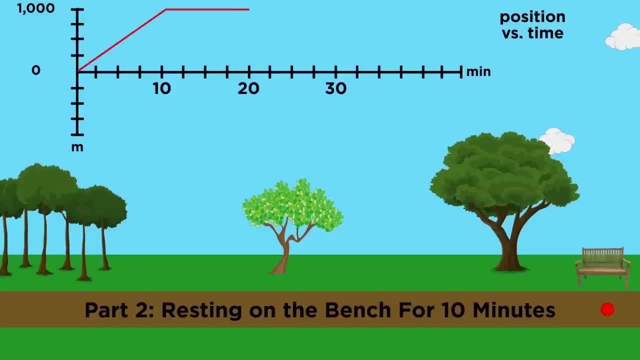 of twenty minutes and one thousand meters. Then, very excited about your pizza, you jog halfway back, or five hundred meters at a rate of two hundred meters per minute. so this should take two point five minutes. This line segment will have a steeper slope because you are covering more distance in. 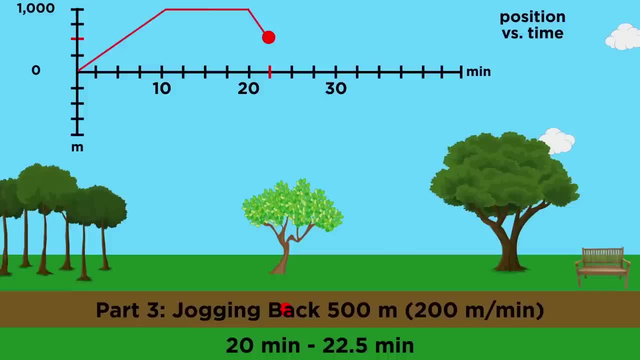 less time and we can see that we are now at coordinates of twenty-two point, five minutes and five hundred meters. Suddenly, you get a cramp and you have to finish the journey at fifty meters per minute, which will take ten minutes, leaving you at a point with coordinates of thirty-two point. 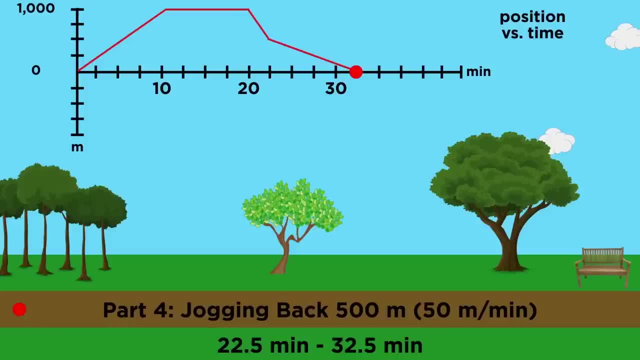 five minutes and zero meters back to the place where you started. but later in time, One thing we will want to be able to do is to take this data and draw a graph for the same activity, but with velocity on the Y axis. 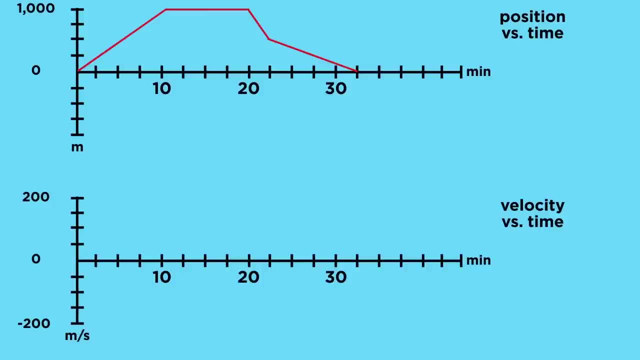 To do this, we just translate each line segment. For the first bit we see that we went one thousand meters in ten minutes. Then we have a point of thirty-two point five minutes and zero meters back to the place where you started, but later in time. 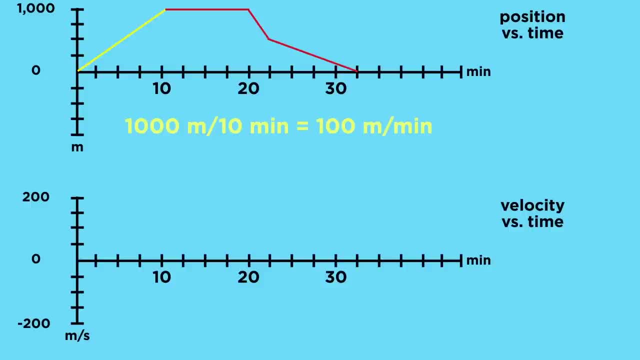 10 minutes, so that's a velocity of 100 meters per minute. So we can draw a horizontal line segment at 100 meters per minute, extending until the 10 minute mark. because you moved with constant velocity during that time. Then you were at rest for 10 minutes, so your velocity was zero. 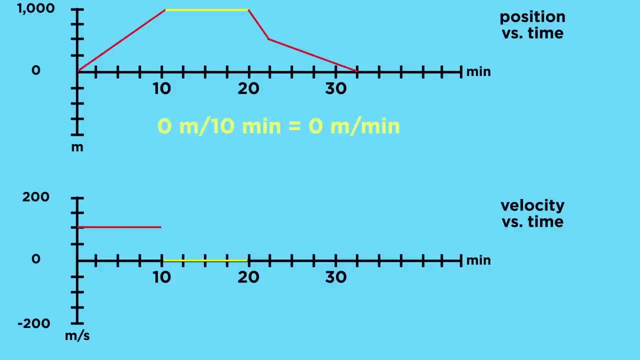 We can draw another horizontal line segment for that time period right on the axis. Then you began moving in the negative direction, so you had a negative velocity. That sounds strange, but remember that velocity is different from speed in that we are also reporting direction. so here, if we went 500 meters in the negative direction over two 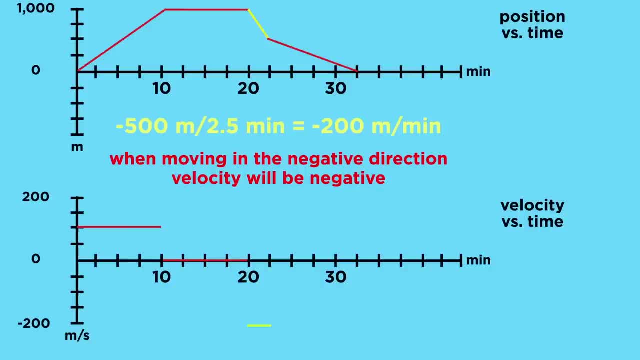 and a half minutes you had a velocity of negative 200 meters per minute, which is down here below the axis. Then for the last 10 minutes, you had a velocity of negative 50 meters per minute. and there is our graph. 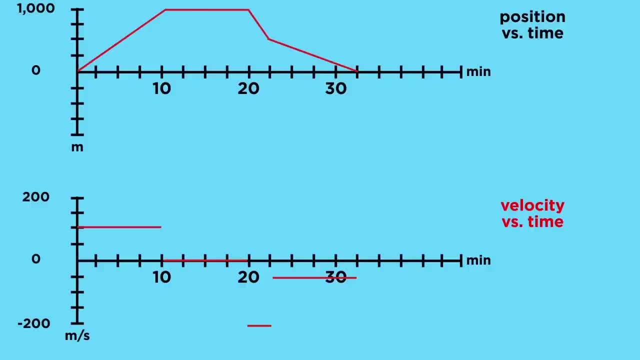 Let's point out a couple things right now. First, we notice that we only have velocity data when the object is moving, When at rest the velocity is zero because there is no displacement over that time period. Also, this is quite oversimplified, because it is impossible to go from a standstill to 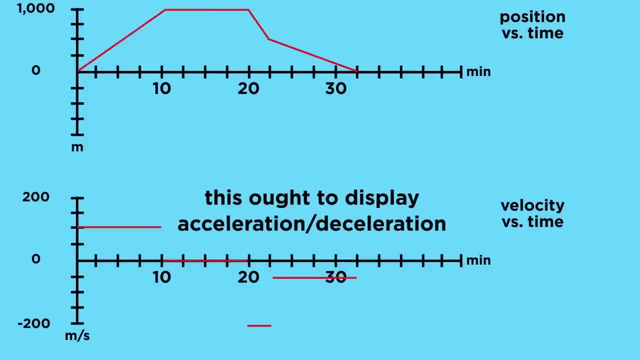 some velocity in an instant. In reality there must be an acceleration or deceleration when starting or stopping. so that means if we were trying to be as accurate as possible, we would quickly ramp up to this velocity and then ramp down to rest, even if it's over just a second or two. 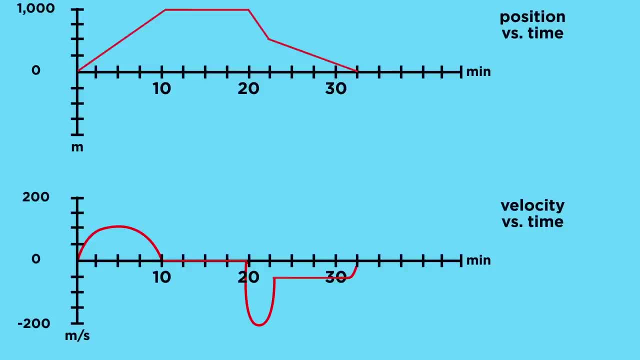 This is important because we will now want to graph acceleration over time And just the way that we can only have velocity data when the object is moving. we can only get acceleration data when velocity is changing, So there will be a positive acceleration as we just start moving. 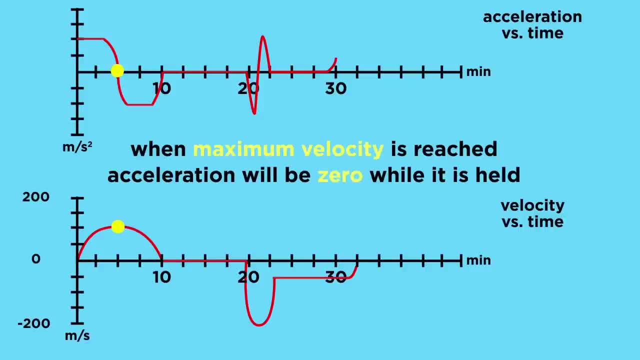 I'll see you next time moving. but it will then come to zero as we walk with constant velocity. Then acceleration will be negative as we slow to a stop. It will be negative again as we begin to walk back, and then back to zero, but then slightly. 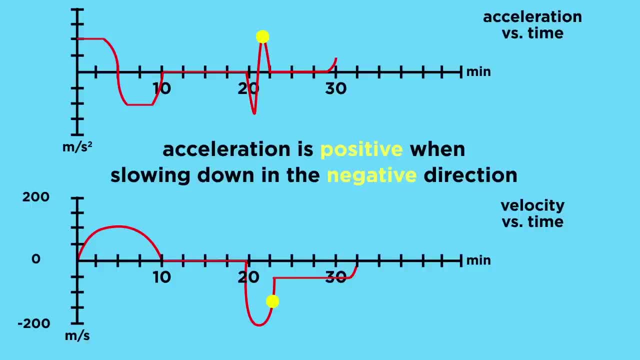 positive when we slow down our movement in the negative direction, Back to zero, and positive again when we stop, as we require positive acceleration to stop moving in the negative direction. We will only have a non-zero value for acceleration when velocity is changing. 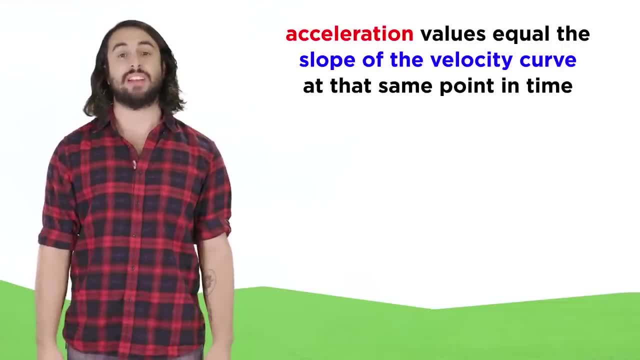 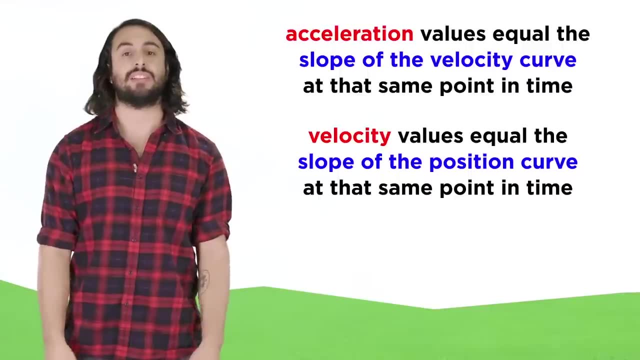 In this way, every point on the acceleration graph is telling us about the slope on the velocity graph for the same point in time, and every point on the velocity graph is telling us about the slope on the position graph for the same point in time. 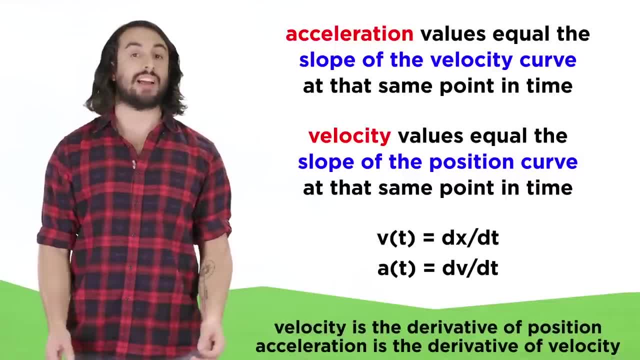 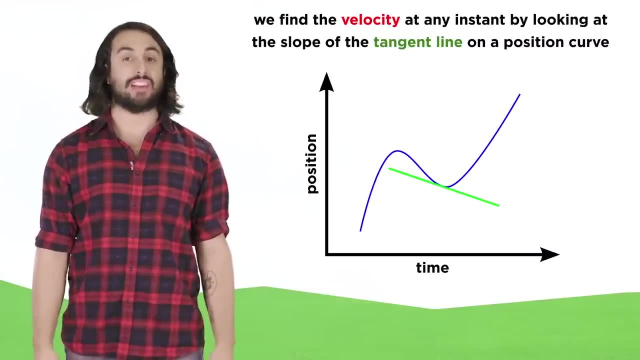 If you are well versed in calculus, you know this means that velocity is the derivative of position with respect to time, and acceleration is the derivative of velocity. This explains why we find instantaneous velocity on a position curve by looking at the tangent line. 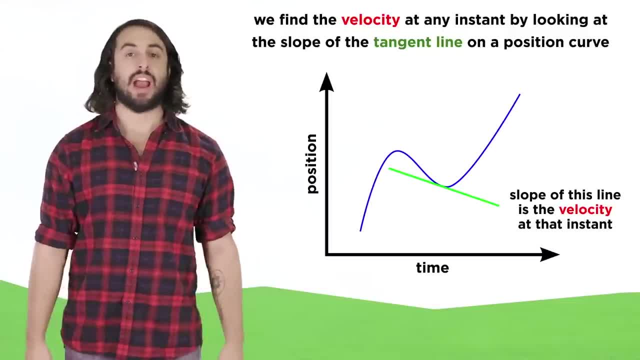 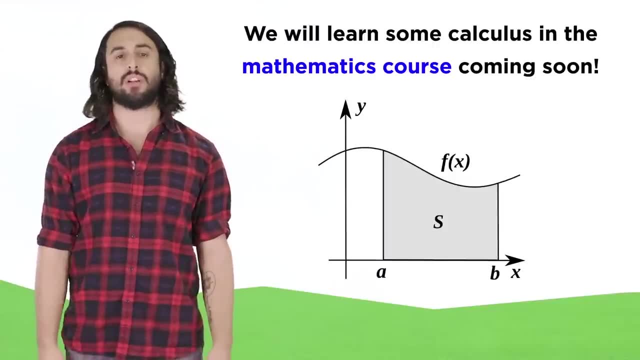 The slope of this line gives us the velocity at that instant, and the slope of the tangent line on a velocity curve will give us the instantaneous acceleration. We will cover all kinds of calculus in the upcoming mathematics course, but for now we are going to stick to physics, without complex math, since we are focusing on basic concepts. 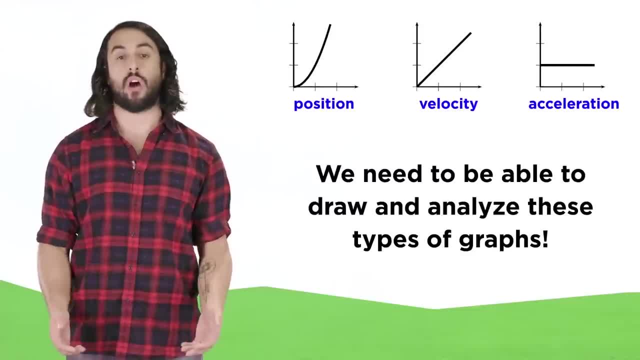 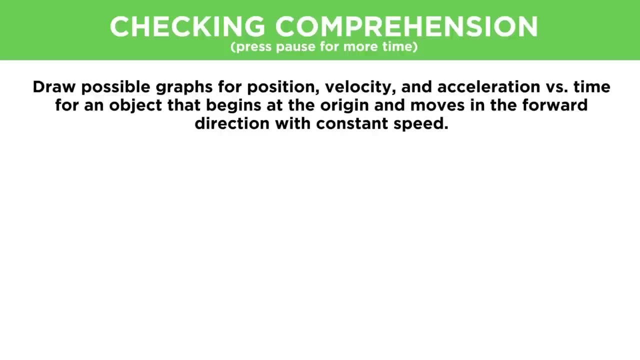